In this video we're looking at finding the nth roots of a complex number which is in polar form. So the question we're going to look at here is using De Moivre's theorem to solve the equation. z to the power of 3 is equal to 8.. Now, before we get into actually solving this equation, I've 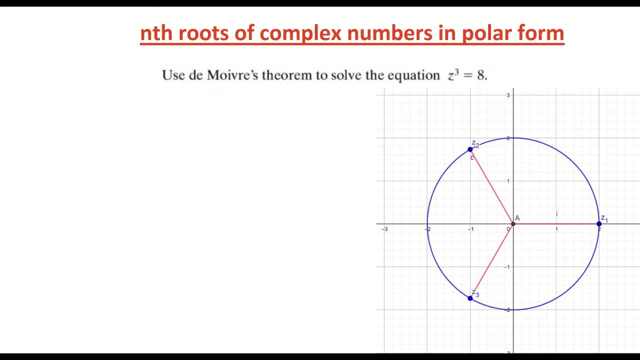 actually put up a diagram of the answers and because the question is to the power of 3, so the complex number z to the power of 3, it means that there's going to be three solutions or three roots, and you can see here that we have the three roots. I've called them z1, z2 and z3. on the 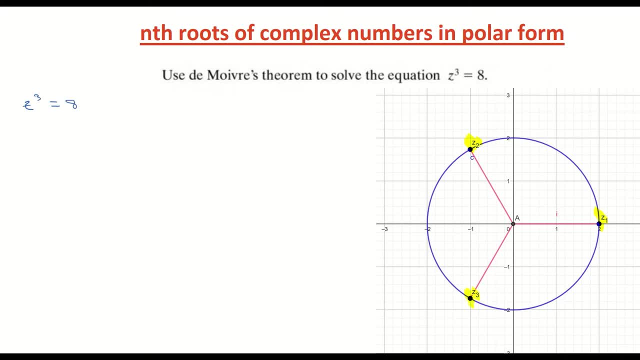 diagram. So that's the first thing I want you to see. When you're finding z to the power of 3, there's going to be three answers or three roots. Now, if this was z to the power of 4, you would have four roots, or z to the power of 2, two roots. You'll also notice that the angle between each of 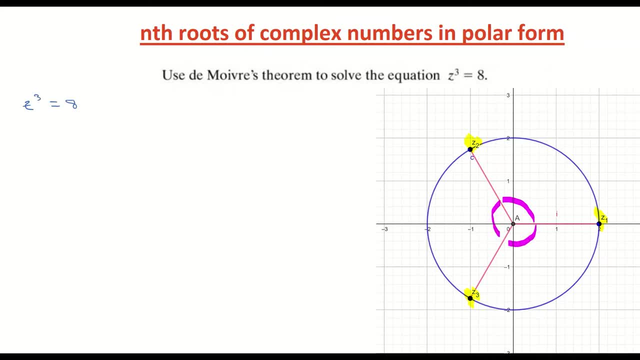 these complex numbers is the same size. so this circle is broken into three segments. So that's just to give you a little bit of background as to what you're trying to achieve here. You're trying to find those three complex numbers. So, as I look at my complex number, 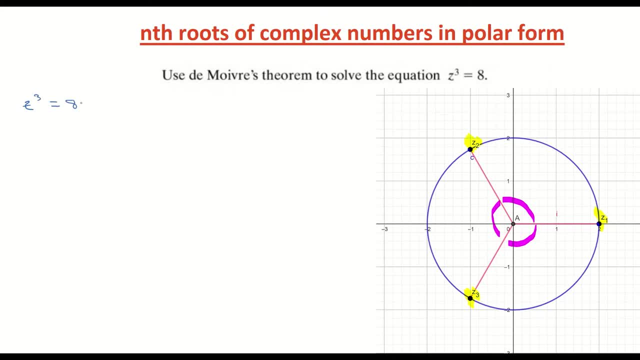 z3 is equal to 8. they've only given us a real part to our complex number, but I'm going to just put in my 0i just to make it easier to work with. So my complex number here is 8 plus 0i. Now that's. 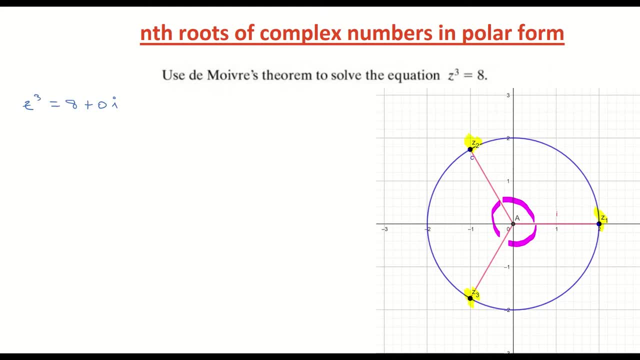 in rectangular form. Let's put that complex number into polar form. So to turn that into polar form, we need to put it into r times cos theta plus i sine theta. So that's the form we want our complex number in and in order to find our r, 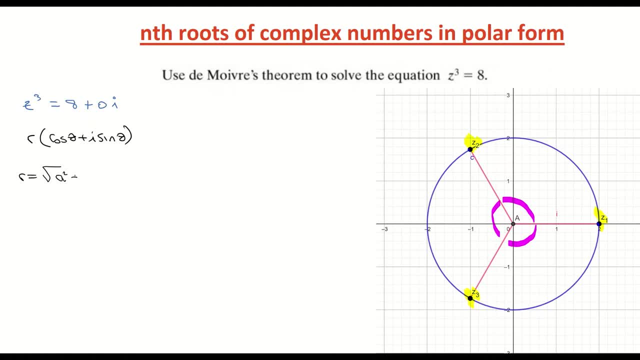 our r is found by getting the square root of a squared plus b squared, and our a is the real part and the b is the imaginary part. So that's my a and my b. The theta, then, is the angle between the x-axis and the actual complex number, and that's found by getting the inverse. 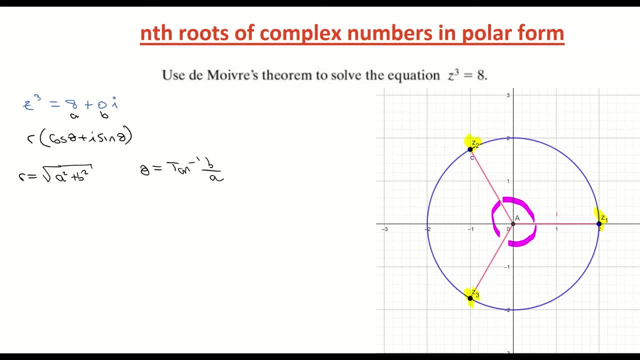 of b over a. So there are the two parts we need. We need our radius, our modulus and our angle, our argument. So if I do a quick sketch of this complex number, 8 plus 0i- So this is my real, this is my imaginary- If I was to plot that complex number it would go roughly around here, That's. 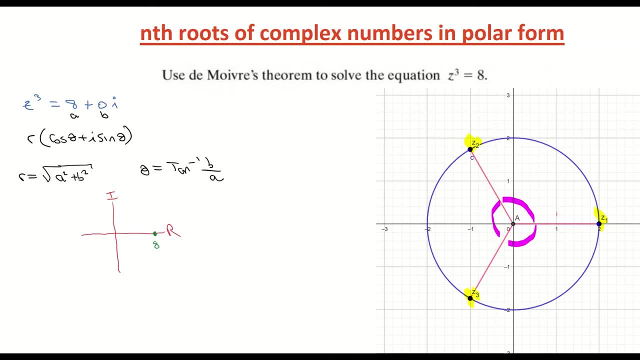 the complex number. So I go out 8 on the real and I go up 0 on the imaginary. So that's the complex number and you can see from that that the modulus of that complex number is in fact fact 8.. We know by looking at the picture it's 8, but let's just use 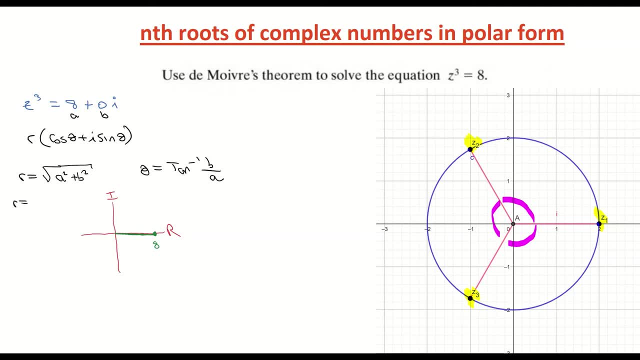 mathematics to get to that. So if we find our modulus, r is equal to the square root of a, which is 8 squared, and b, which is 0 squared, and that's giving me. then r is equal to the square root of 64. so r is equal to 8, and lo and behold. 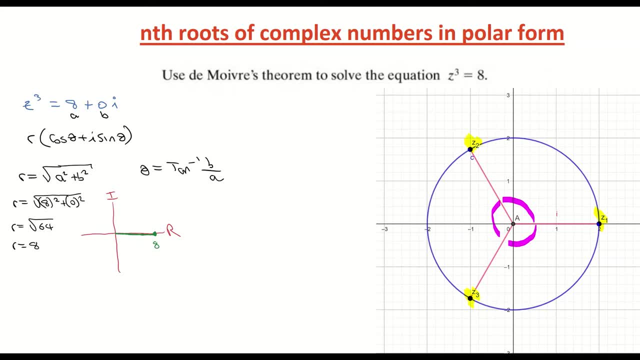 that's what we basically marked on our picture. You can also see on the picture what's the angle between that coordinate, that point, and the x-axis. Well, there is no angle. it's 0, it's right in here. The angle there is in fact 0, and if you were 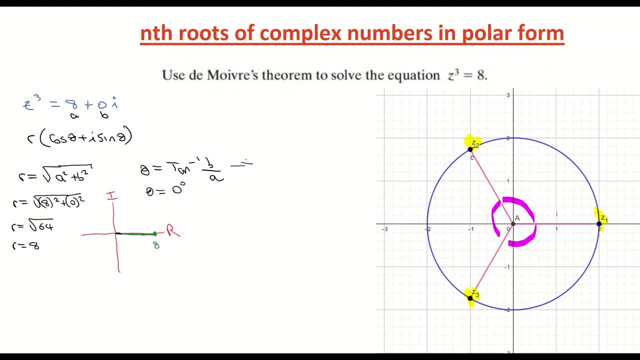 to go to your calculator and actually do this using our tan inverse, you will notice that you'll get tan inverse of b over a, which is 0 over 8, and if you put that in on your calculator, it will also come up as 0. So, as I said, you can either. 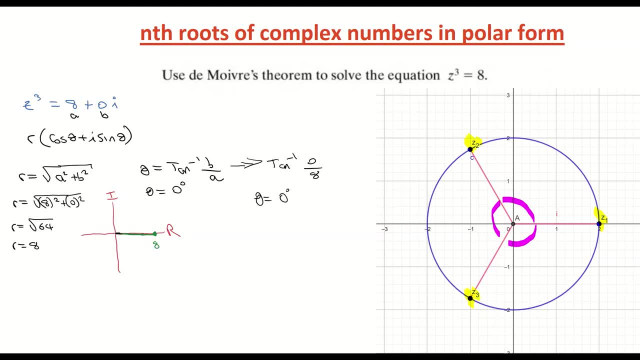 use your knowledge of sketching or you can use your two formulas. Now, that's 0 degrees, which is the same as 0 pi if we're working in radians or degrees. So we have 0 degrees or 0 pi. So filling in my complex number, that's. 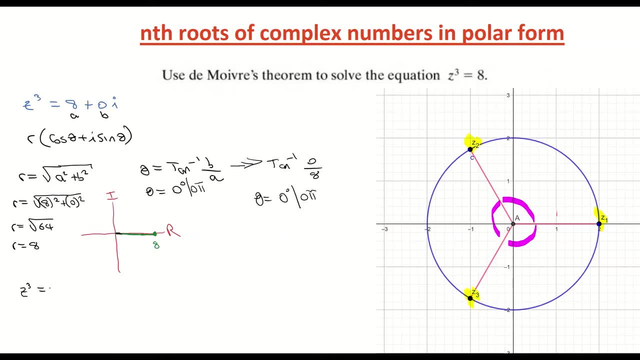 giving me z to the power of 3 is equal to r, which is 8 times cos theta, theta being 0 pi plus i sine 0 pi and close my bracket. So there's my complex number. Next thing I want to do is to eliminate. 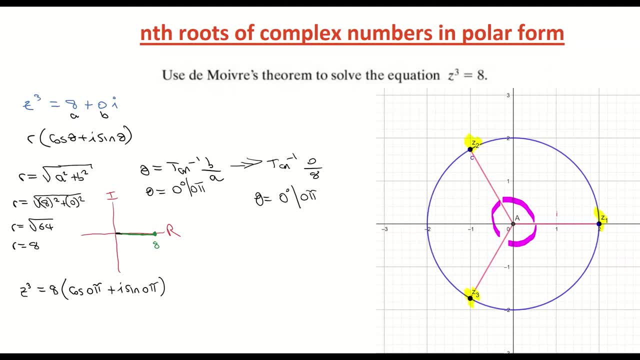 this power of 3.. So if you think about a number, let's just pick the number, like 8 itself. If I was to get the cubed root of 8 on your calculator, you will see that your answer is 2.. Now that's the same as going 8 to the power of 1 over. 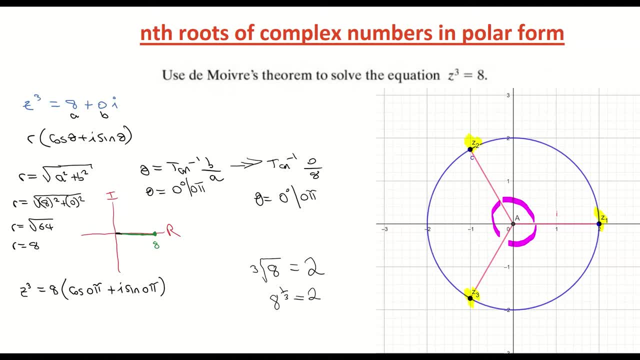 3.. So that's the same thing. That's what the cubed root is doing. It's putting it to the power of 1 over, and that's what I'm going to do here, to to get rid of that z to the power of 3.. I'm going to basically multiply across by the power. 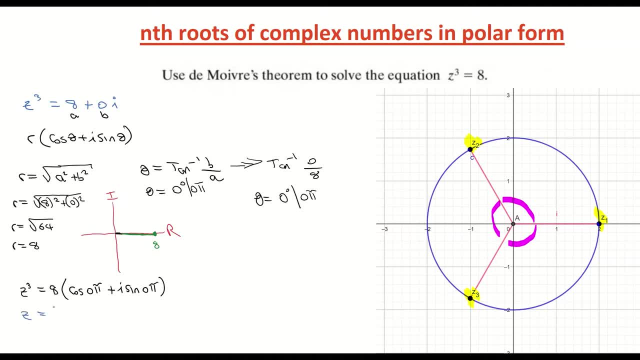 of 1 third. so that means then that z to the power of 1 is going to be 0. Now, if you is equal to 8 times cos 0 pi plus i sine 0 pi, and it's all to the power of 1 over 3. 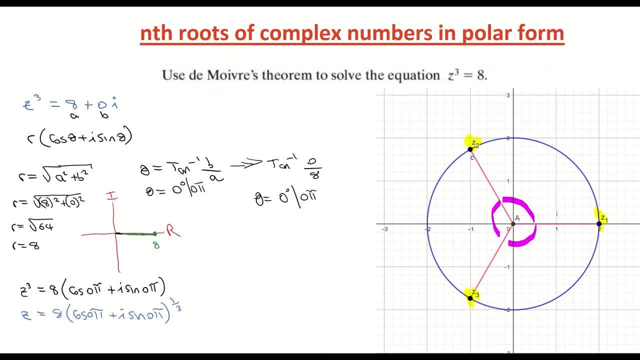 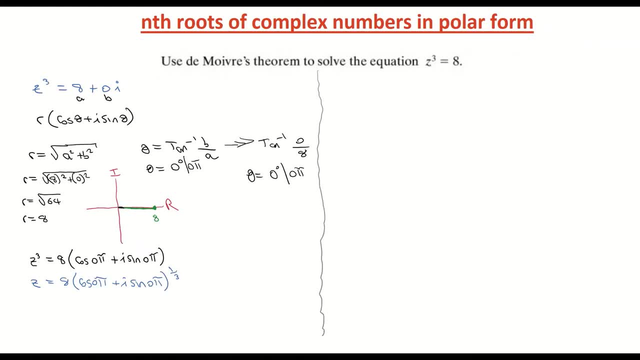 and that's the same as getting the cubed root, basically. so that's our complex number in polar form. so I'm just going to write that in here. so this is in polar form. now what I want to do is I want to write this complex number in. 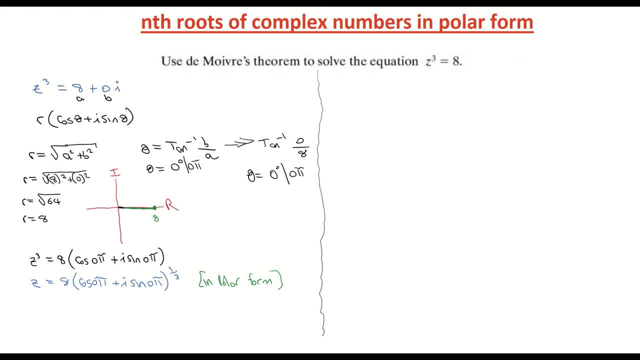 general polar form. so basically what we can do is, if you think about it, if I've just taken out that circle now, but that circle rotates in 360 degrees, or 2 pi is the same as 360 degrees. so every time I go around, 2 pi or 360 I'm bringing. 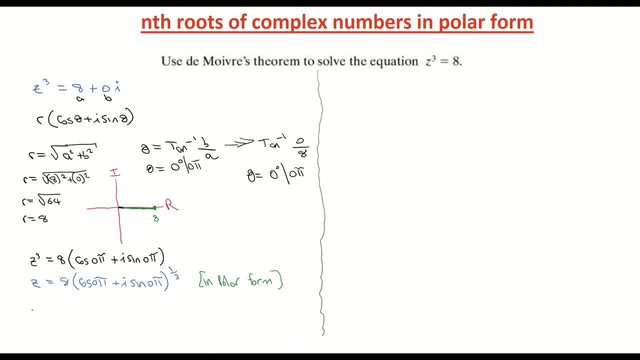 myself back to that original complex number. so that means that I can rewrite Z, as Z is equal to 8 times cost 0 pi. so that's what I have in my polar form. but what I'm going to do here is I'm going to add on 2 pi and I'm going to add on 2 pi n and n stands for 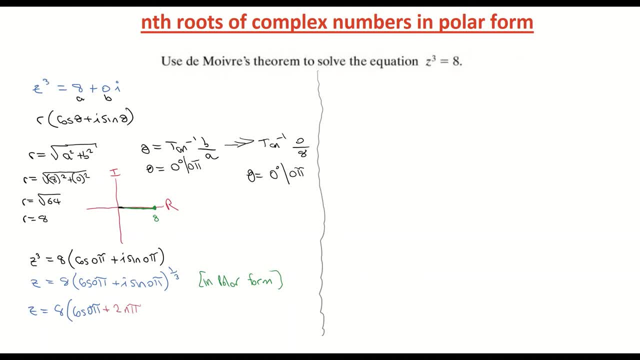 a number of circles or a number of rotations, so I could go around once, twice, twice as many times as I want. so that's what the n stands for. so I'm adding on that 2 n pi onto my angle and because I'm doing it to the cos I need. 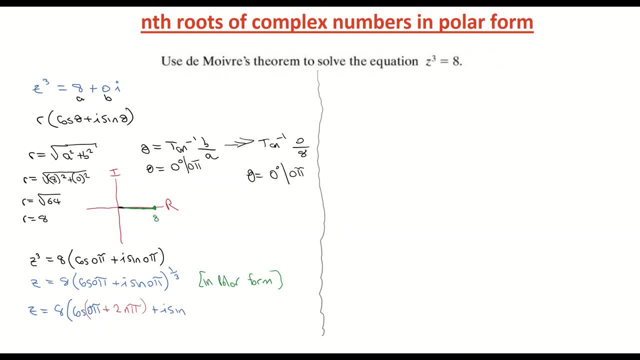 to do this. It's difficult to learn the derivative from a smaller derivation of a moab equation, so I'll do it later, at next half minute. to the sine. so that's plus i, sine, zero pi, plus two n pi. so again, that is just standing for the. 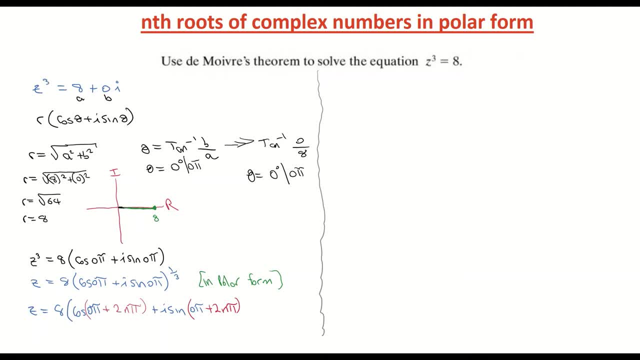 amount of rotations that i'm doing and i'm going to close my bracket, and again, that's to the power of one third and that's basically known as my general polar form or the general form. so we would have looked at this in trigonometry as well. so now i'm going to use my knowledge of 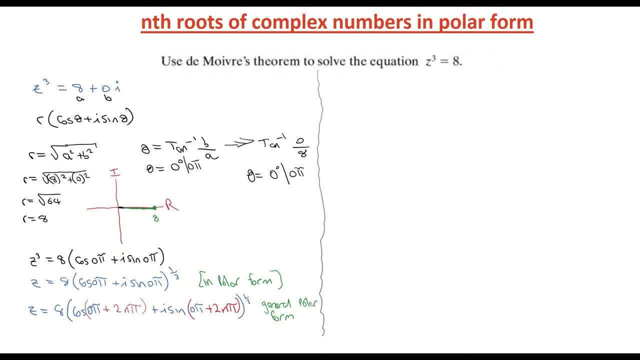 de moivre's theorem to deal with the power. so how do i deal with the power? i put the or to the power of the one third. so that's my first step. so i'm writing now: z equals eight to the power of one third. so this is coming from my 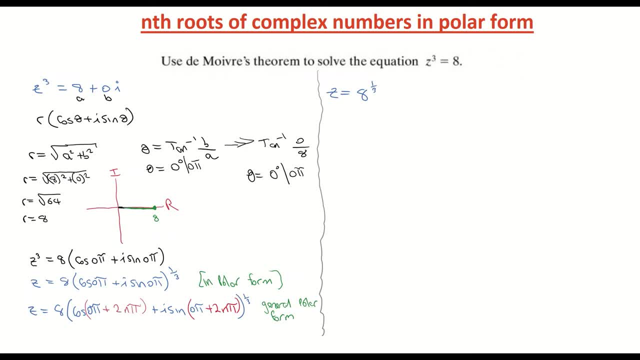 de moivre's theorem, and that then is times cos of my power, which is one over three, and then i'm then multiplying that by my zero pi plus two n pi. plus i sine one over three times zero pi plus two n pi. so that's, using my de moivre's theorem, 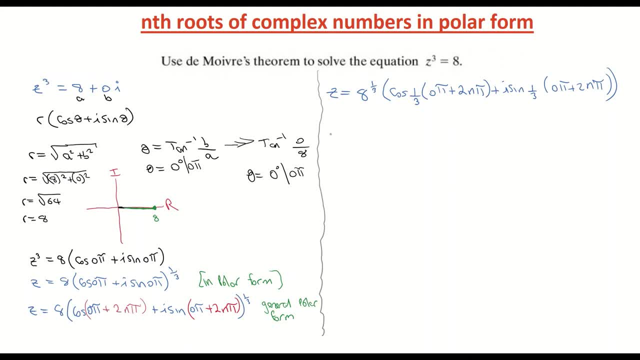 and i'm now going to evaluate that. so what does that give me? eight to the power of one third is two, and pi cos cosh one third. well, let's just focus in on what's inside the bracket here. first, zero pi plus two n pi. well, 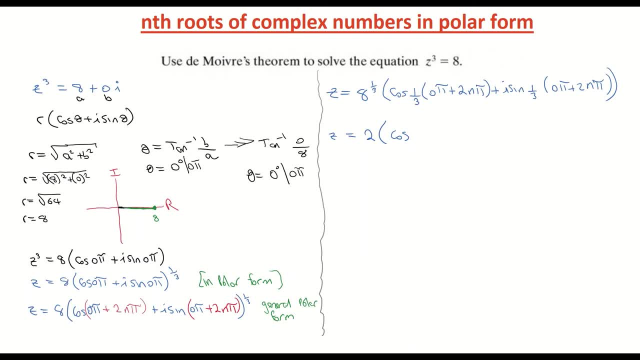 that's just going to leave me with two n pi, so let's write that in first. so cos one third times two n pi, plus i sine one third times two n pi, so it's the same thing. next thing i'm going to do is i'm going to actually multiply in that one third, so i go two. 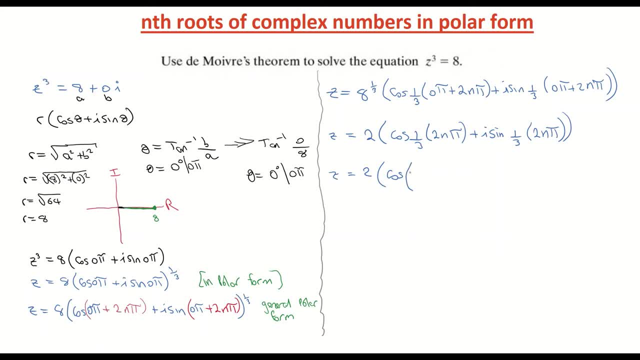 times cos. multiply in the third. you don't have to do this step, but i'm just going to multiply it in as a single fraction. so top by top, bottom by bottom will give me 2 n pi over 3 plus i sine 2 n pi over 3. so there's my complex number in polar form, that's. i've now rewritten z as equal. 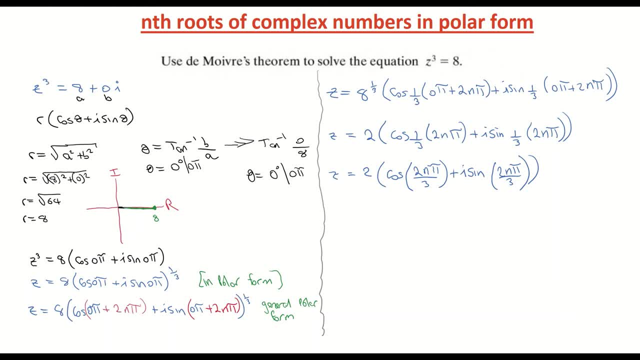 to that. now what i have to do is basically find the three roots because, again, if we focus back on the question, they wanted it to be z to the power of 3. now there's three roots. the first root we have to be careful with here. in order to get the first root, we're going to sub 0 in for n. 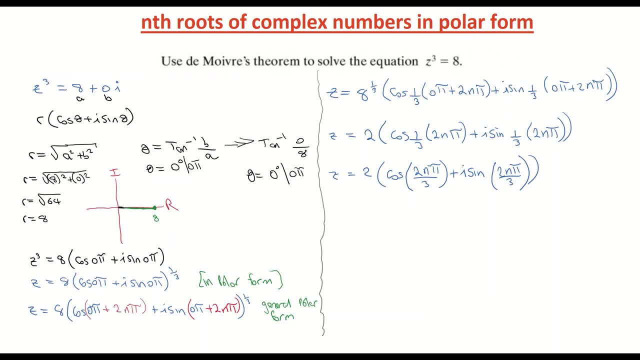 because, just think about it, we're not actually going to go within a full rotation of my circle, so that's why i'm staying at 0. so the first thing here i'm going to do is: let n is equal to 0, so i'm going to solve when n is equal to 0. so that's going to give me z is equal to 2 times cos. 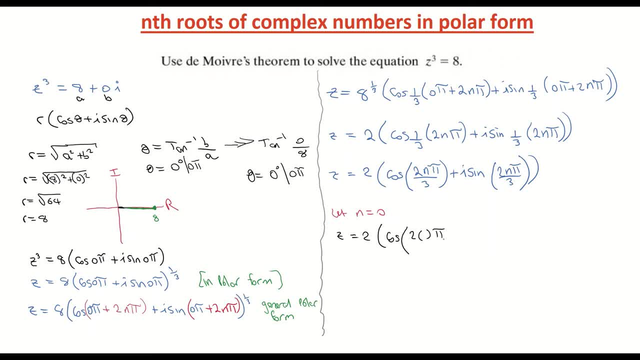 2 times 0 pi over 3. so i'll come back and i'll sub in that 0 now in one second. plus i sine 2 times 0 pi over 3, so i'm basically, as i said, subbing in 0 for n and when i evaluate that i get 2 times. 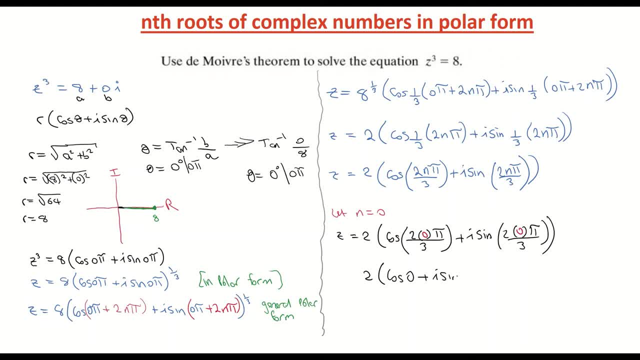 cos of 0 plus i sine of 0, and when i go to my calculator and i type in cos of 0, pi, i get 1, and when i type in sine of 0, i get 0, so that becomes 0 i. and now i'm going to multiply in. 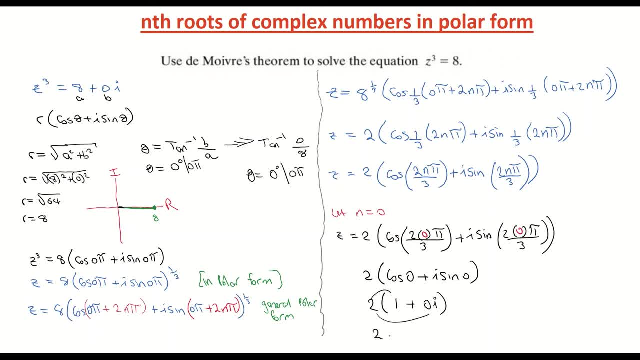 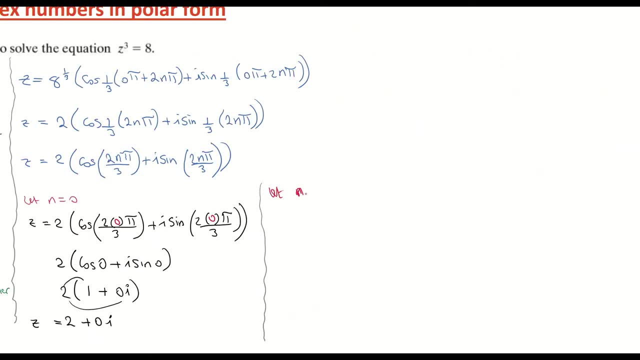 that 2, which is giving me 2 plus 0 i. so there's my first solution: 2 plus 0 i, or just 2. now i'm going to go over and i'm going to do: n is equal to 1. okay, so it's the same system. again. i'm going to go. z is equal to 2 times cos of. 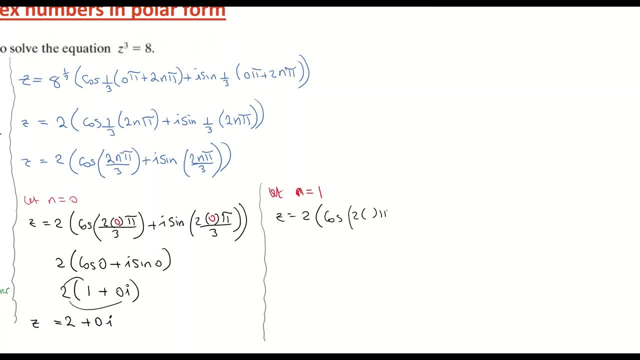 2 times 1 times theta again. i'll come back in a second and i'll fill in that 1 in red plus. i sine 2 times 1 theta over 3 and i'm closing my brackets, i'm putting in my 0 and i'm going to. 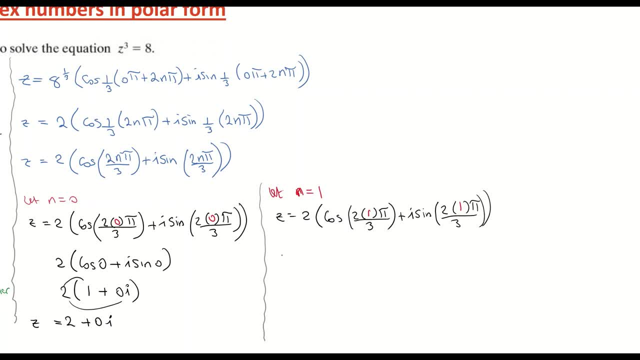 put in my 1. now when i multiply in my fractions i'm getting: z is equal to 2 times cos of 2 by 1. by pi is 2 pi over 3, plus i sine 2 pi over 3 when i go to my calculator and i evaluate cos. 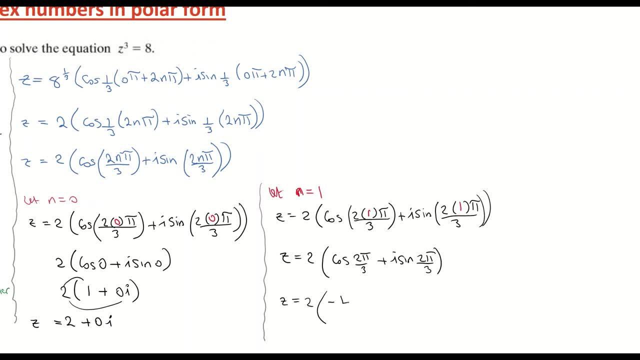 2 pi over 3, i get negative a half. and when i evaluate sine 2 pi over 3, i get positive. root 3 over 2, and don't forget to put back in our i. next step is multiply in your 2, so that's giving me a complex number of. a root of z is equal to 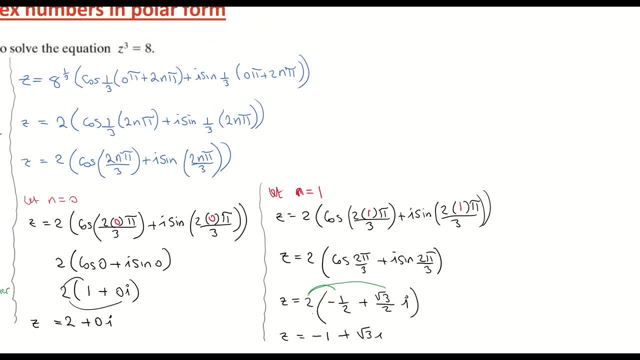 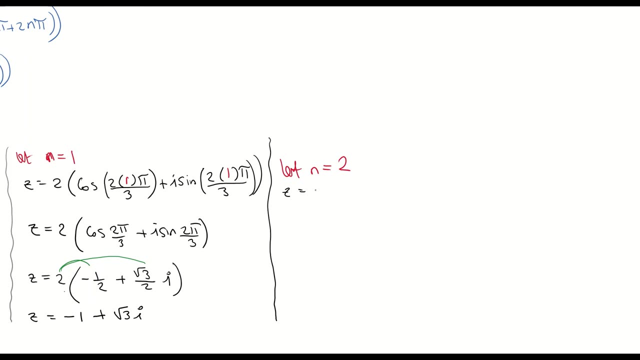 minus 1, plus root 3, i. so there's my second root. when i let n is equal to 1, don't forget, we have three roots here, so my final one is going to be: by letting n is equal to 2, we have z is equal to.